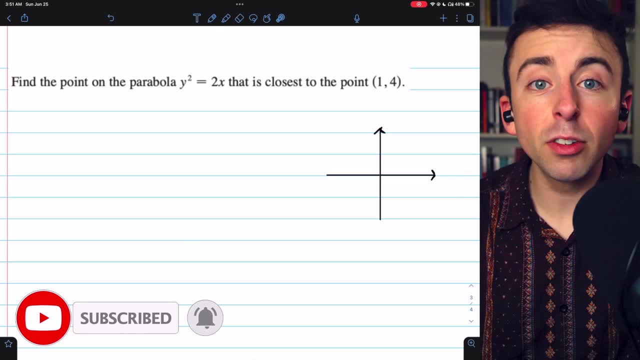 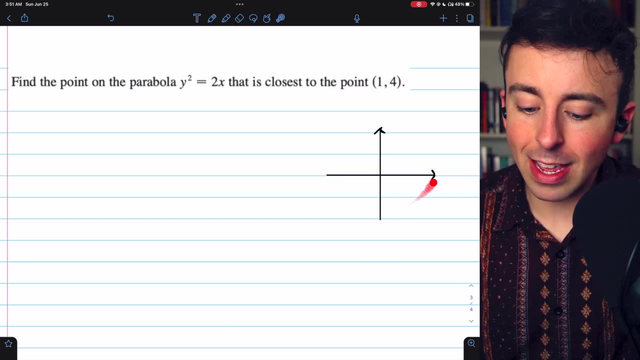 equals 2x. that's closest to the point. So we're trying to minimize distance. Closest right We're minimizing distance. Let's begin with a sketch. Here's the xy plane and we want to graph: y squared equals 2x. y squared equals 2x looks a lot like y equals x squared, except. 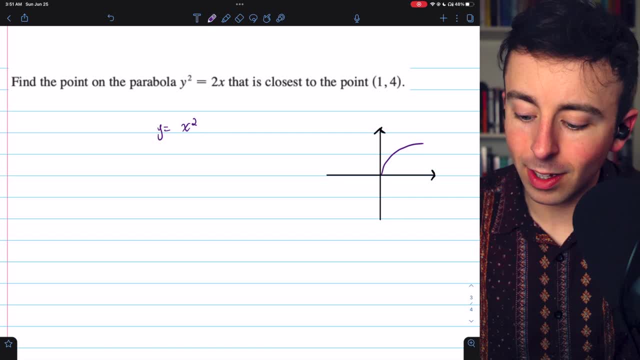 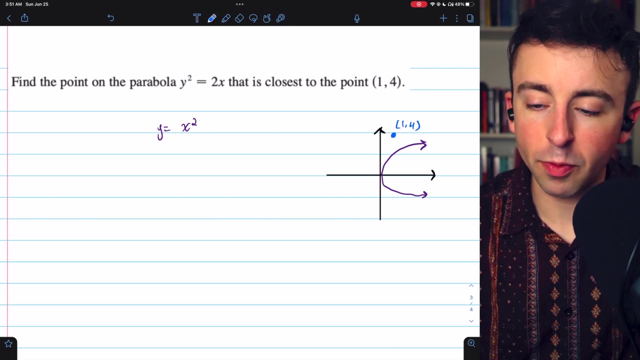 instead of opening along the y-axis, it opens along the x-axis. The specifics of the sketch aren't too important And let's say the point is maybe right here and we're trying to minimize the distance between the parabola and this point, Or rather we're trying to find the point on the. 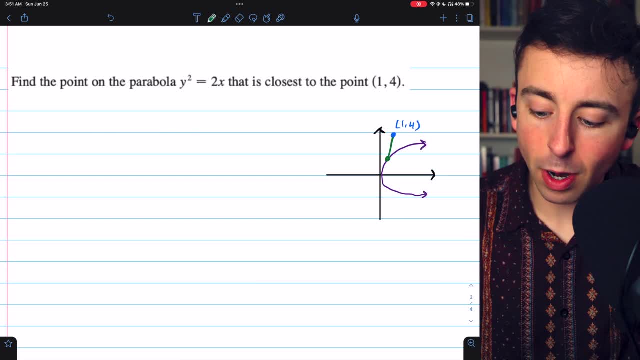 parabola with minimum distance And if the point is scheduled for the left side or the right side of the parabola, We want to. Any point on this parabola has some distance from the point. we're trying to find which point is closest. 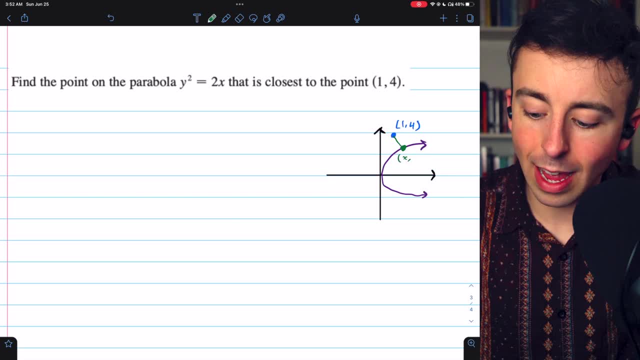 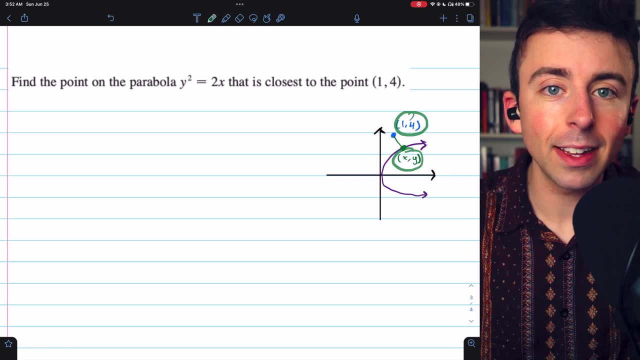 So let's just sketch a point on the parabola, say it has coordinates, The distance between a point on the parabola, and is what we're trying to minimize. We'd also want to write our secondary equation, if there was one. 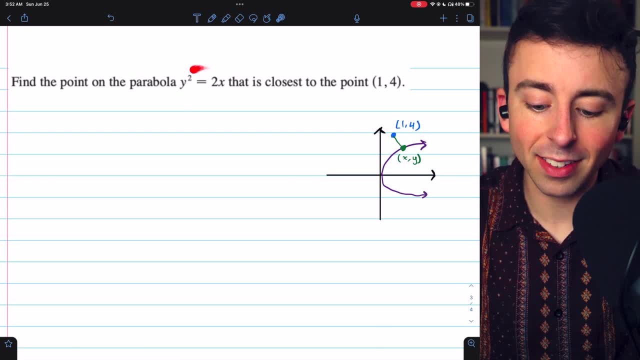 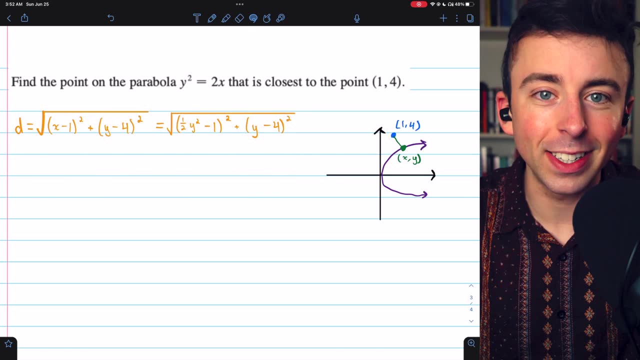 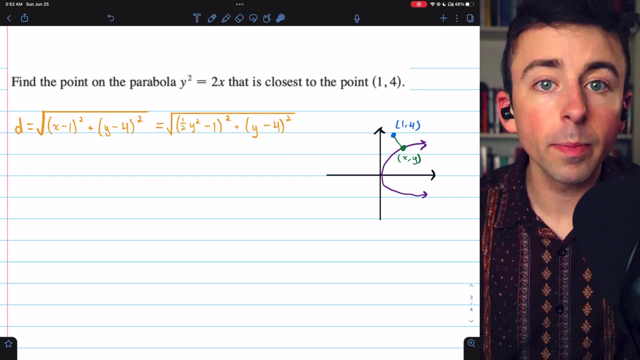 There is one, but it's already written for us: y squared equals 2x. That relates x and y, and that's going to come in handy for writing our primary equation, which is the equation for distance. This is the distance between any point on this parabola and the point. 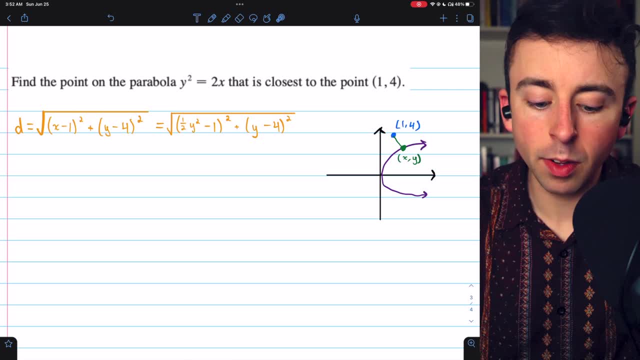 It's the familiar distance formula. We have the square root of x minus 1 squared, that's the difference in the x coordinates squared, plus y minus 4 squared, the difference in the y coordinates squared. Again, this is just the distance. 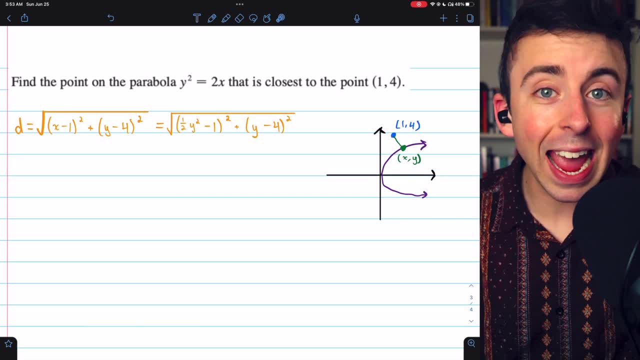 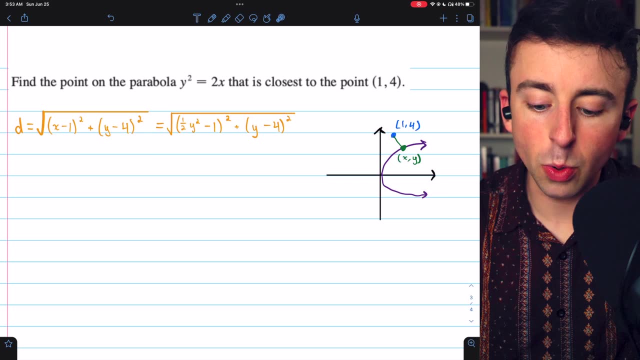 The distance between an arbitrary point on the parabola and the point. To put this equation in terms of a single variable, well, we know that y squared equals 2x, which means x equals 1 half y squared. So where we had x, we'll just put 1 half y squared, giving us this equation for distance. 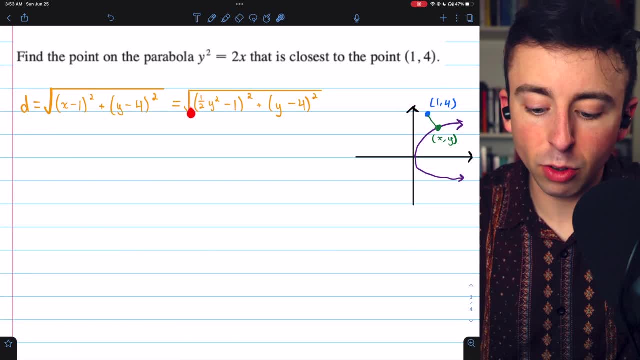 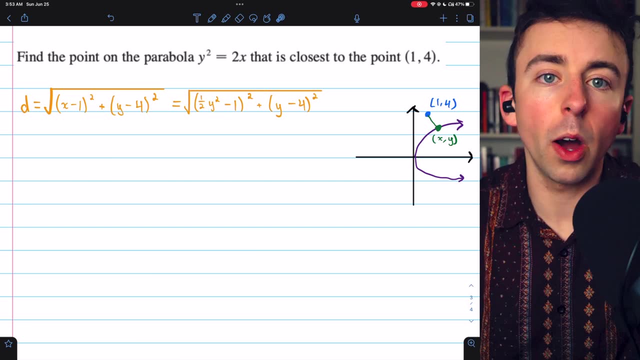 in terms of a single variable. We could move forward using this square root function for our distance. However, the distance we know is going to be positive. Right, The square root always gives a positive number, And x squared- or we could say d squared in this case- is increasing whenever d is greater. 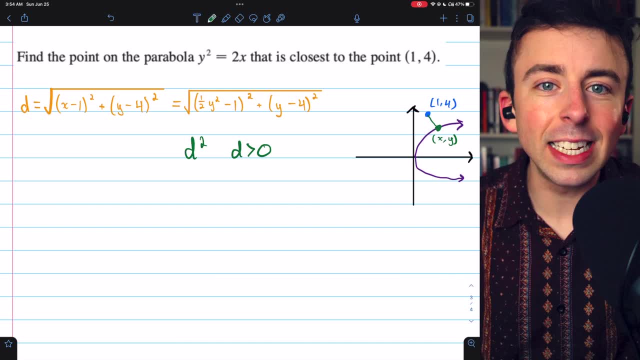 than 0, which means wherever d squared is smallest is also where d is smallest. So the minimum of d, which is what we're looking for, will also be the minimum of d squared. So it would actually be easier if we just worked with d squared. 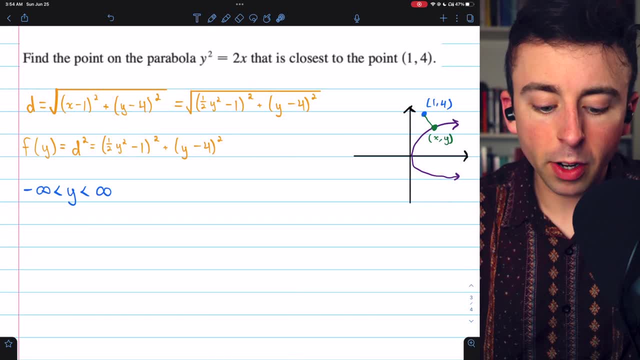 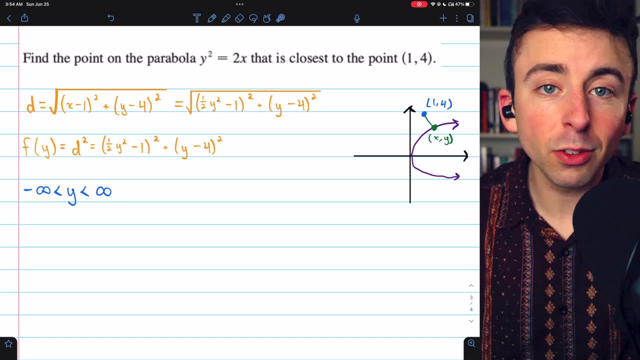 That way we don't have to deal with the distance, We don't have to deal with the messy square root. So we'll call our function f of y. What f of y is is d squared, which is just the distance function, but without that square. 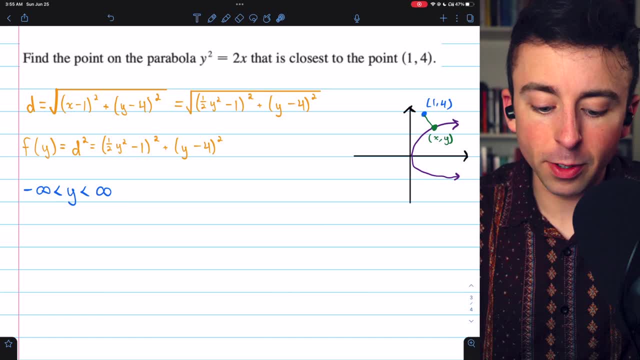 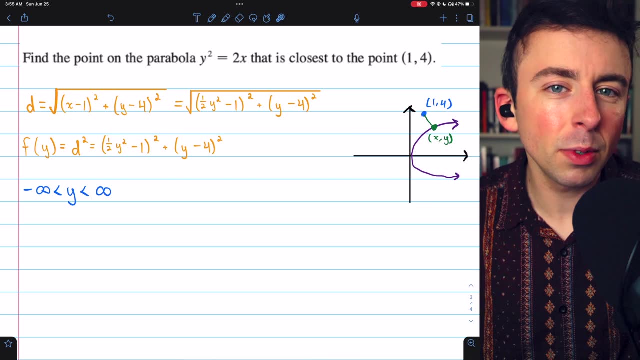 root because we squared it Again. the idea is that wherever d squared is minimum, that's also where d's minimum occurs, So this one will be easier for us to find because we don't have to deal with the square root. We also need to identify the domain of our function. the allowable values for y. 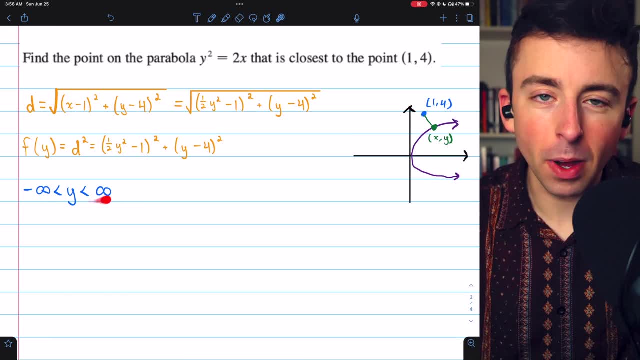 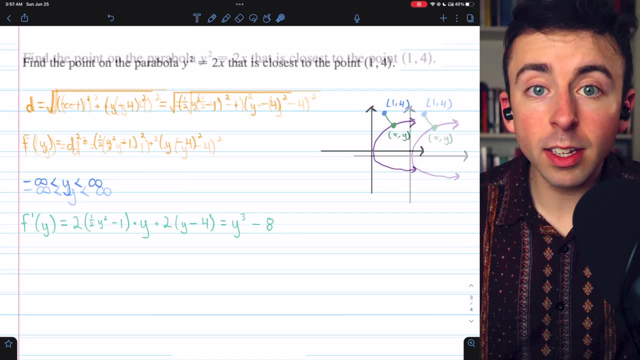 In this case, y could be anything From negative infinity to positive infinity. This is a geometric situation, so there's no real-world restrictions. Y could be anything. Since we're not focused on a closed interval, we will have to use the first derivative test. 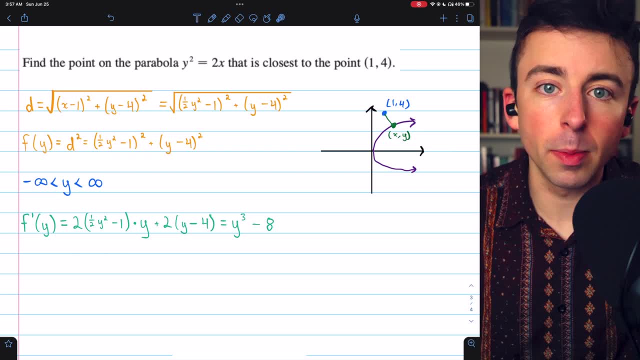 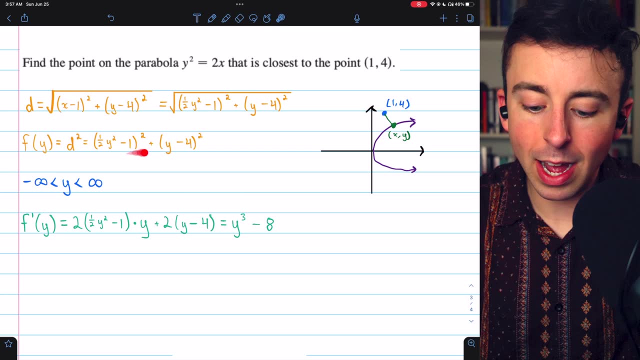 or second derivative test to classify our critical points as minimums or maximums. We, of course are looking for a minimum, But let's get to it. We'll take the derivative of f of y and then we can find our critical points. 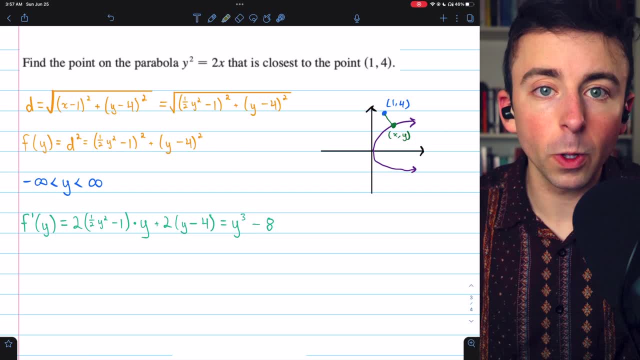 To take the derivative of this, we're going to have to use the chain rule, And that gets us here. The derivative of a thing squared is just 2 times that thing, But then we need to multiply by the derivative of the inside function. 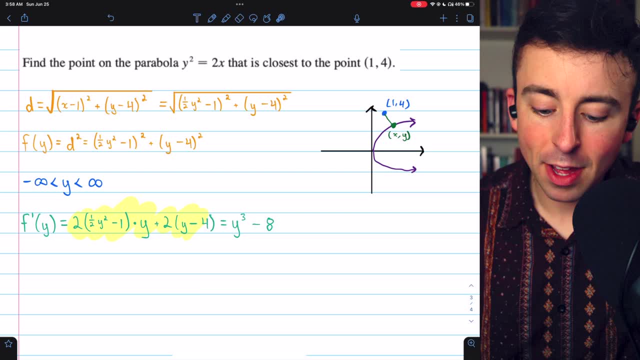 The derivative of 1 half y squared is just y. Then the derivative of y minus 4 squared is similar. The derivative of a thing squared is 2 times the thing Multiply by the derivative of the inside function. In this case that's just 1.. 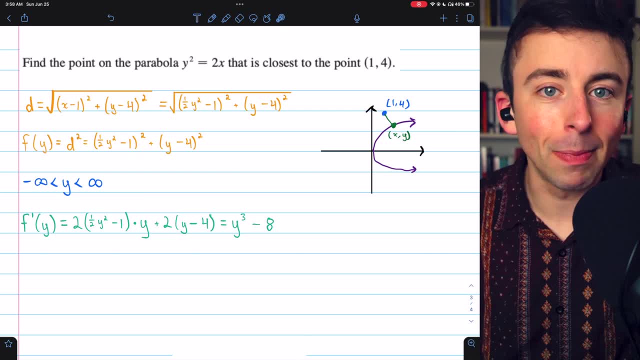 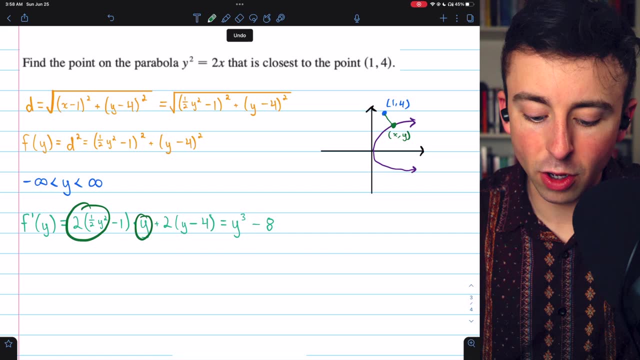 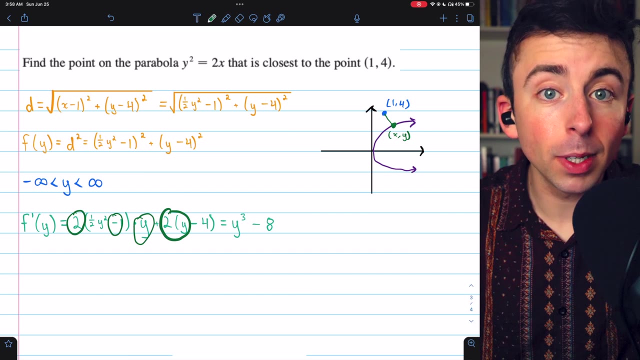 Now, if we simplify this, we end up getting y cubed minus 8.. That's because 2 times a half y squared is y squared Multiplied by y gives us y cubed. But then 2 times negative, 1 times y is negative 2y, which cancels out with that plus 2y.